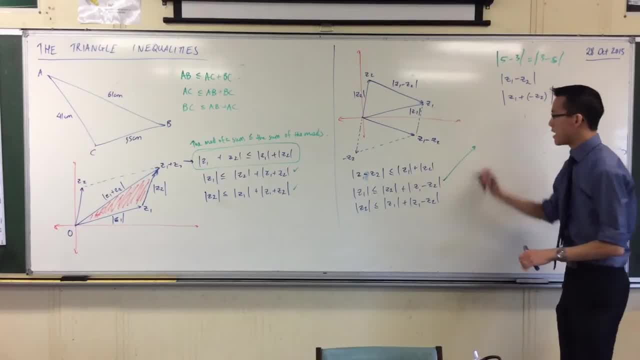 In fact, I'll take the bottom one and I'll show it with that as well, But for now I think it'll be most direct with the middle one. okay, So let me show you. Excuse me, The first thing I'm going to do is: you can see I've got. 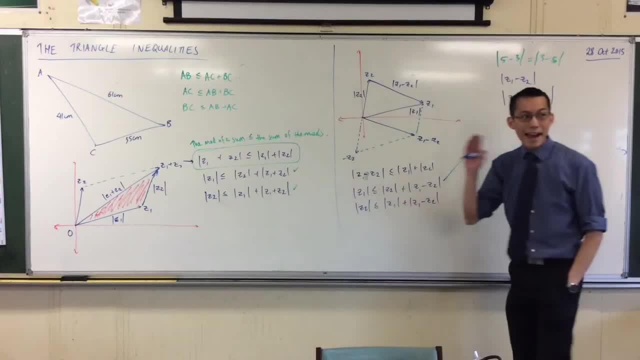 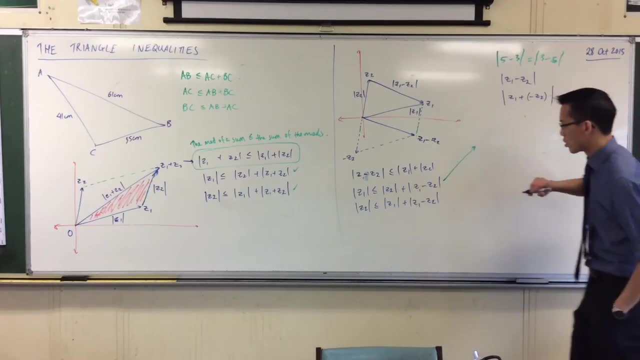 I've got an order here: z1, z2,, z1, z2,. okay, I have the same order in here, if all I do is a tiny little bit of algebraic adjustment, okay, So what I'm going to do is I'm going to subtract z2.. 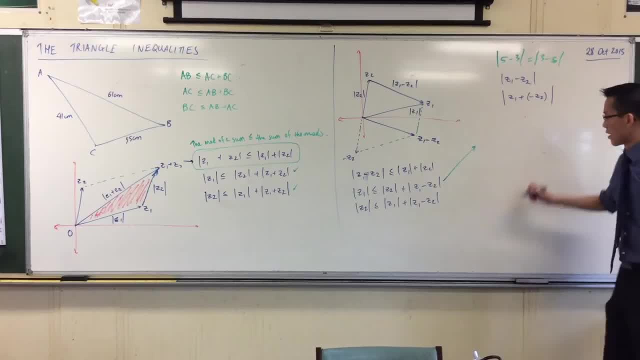 I should say the mod of z2.. I'm going to subtract that from both sides, okay? So here's what I get, Okay? Well, all I've done is subtract mod z2 from both sides. okay, Now, in order to get that, 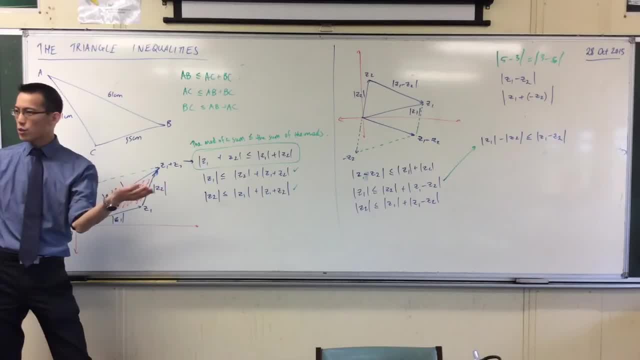 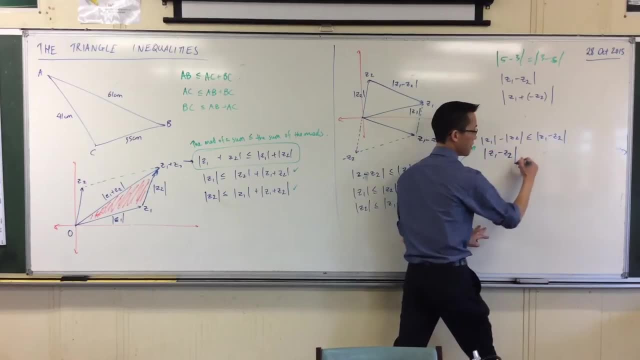 into something that looks a little more like this: I'm just going to flip around the inequality. You see that? So if I put mod of z1 minus z2 there, the modulus of the difference on the left-hand side, then now my inequality switches around. 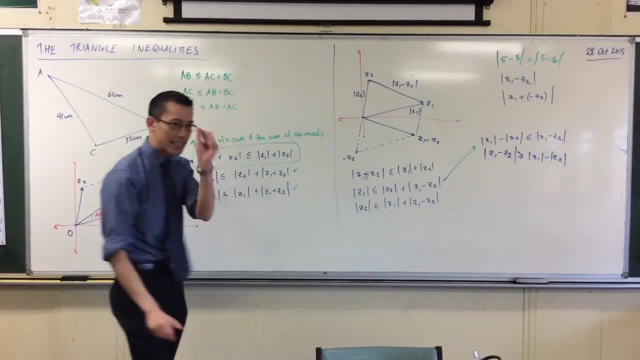 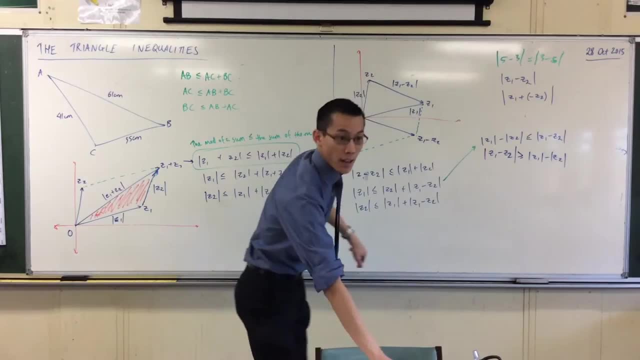 Are you happy with that? Now, how would you articulate, just like I articulated here, how would you articulate, this inequality? What is this in here? Yeah, The mod of the difference is the difference of the mods. Okay, but I'm going to start the same way. 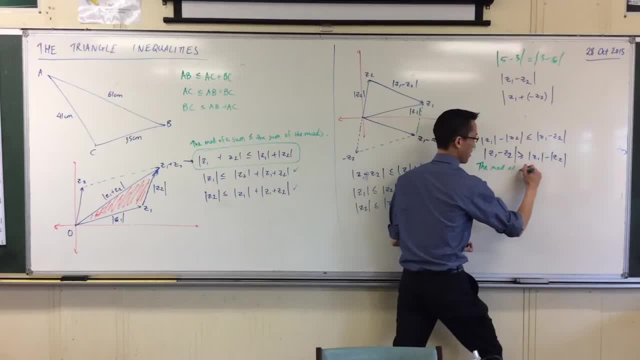 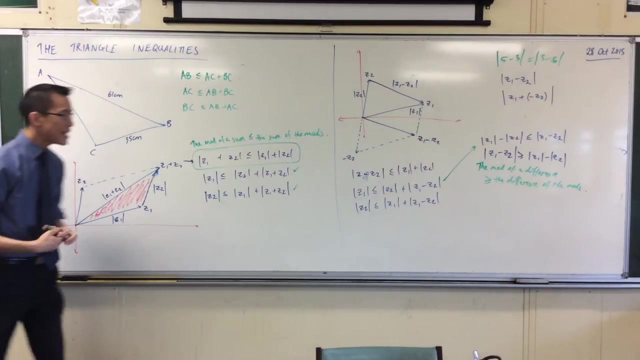 The mod of the difference Is less than or equal to the difference of the mods. Very good, I'll put it here So you can see how this line here we just stated and I'll put a box around it now I'm ready to use it. 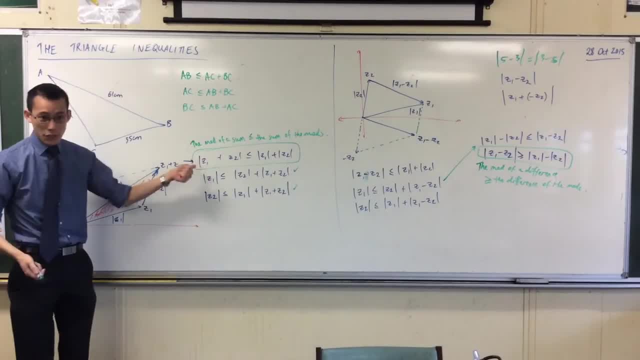 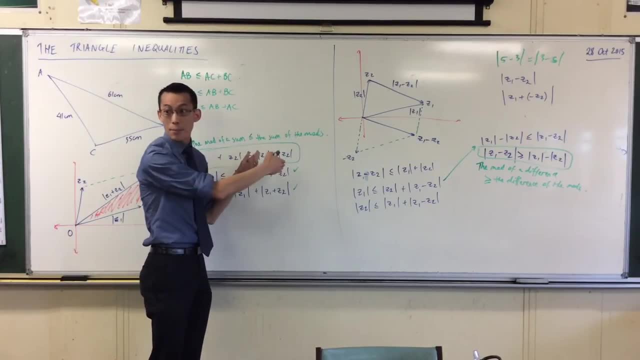 So this statement is kind of like the flip side of this guy. right, If you take, If you add up two complex numbers and take their modules, you'll get something less than the individual module I've taken separately. If you subtract two complex numbers. 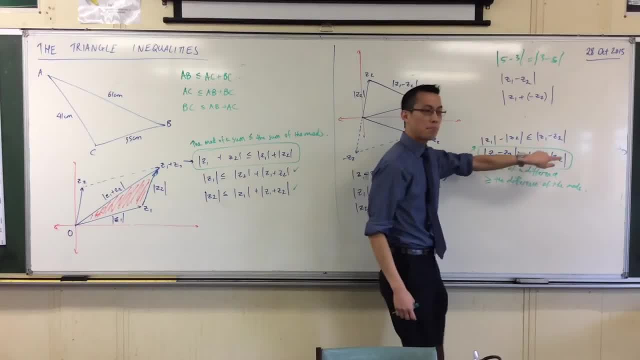 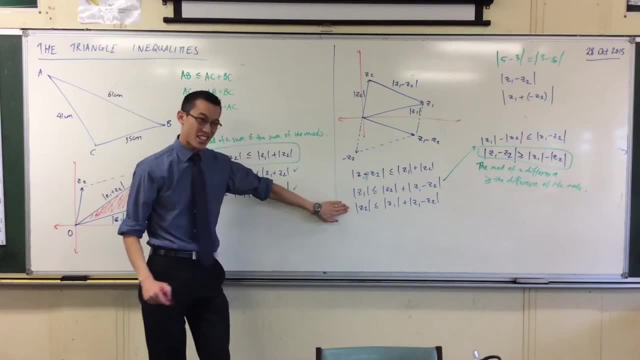 Interesting. If you subtract two complex numbers, you'll get something bigger than if you subtracted the individual ones. Okay, Now, if you remember I said I could have taken this one, I can take this one as well. You don't have to worry about this, but just watch. 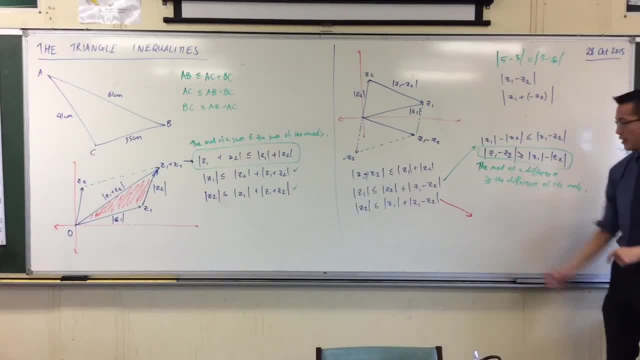 I'll show you If I do the same thing here. right, If I go subtract to get the order thing happening, I'll get Z to take away Z1. on this side, Inequality is still facing the same direction, And then you've got the mod of the differences there. 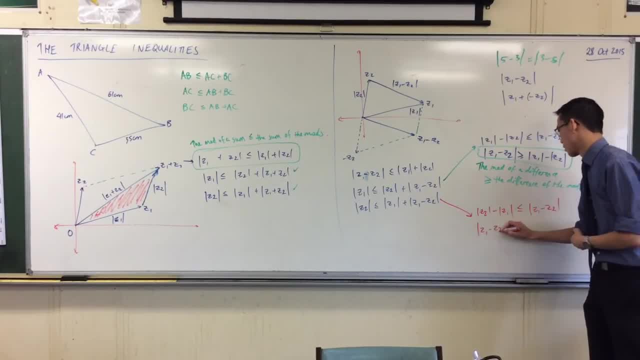 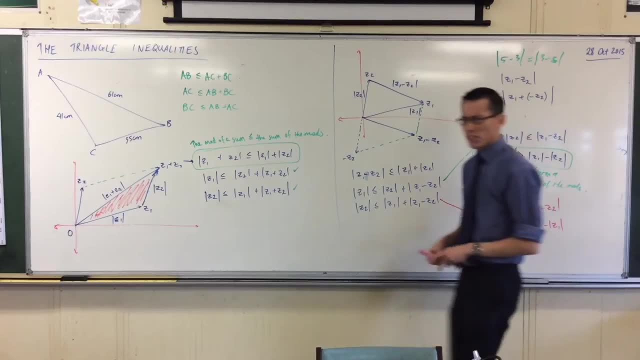 Now, if I switch things over, the inequality goes Careful, because the order matters over here on the right-hand side. And you look at that and you're like, hmm, Like it's almost right but it's not quite. 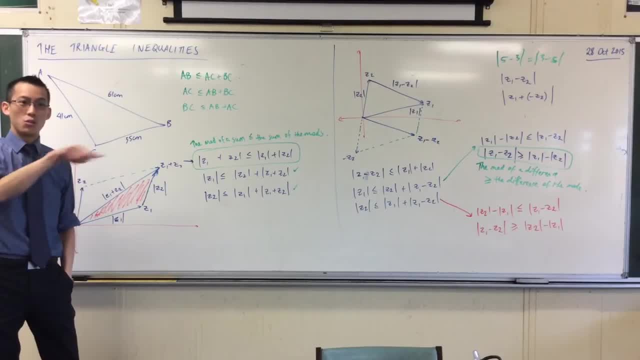 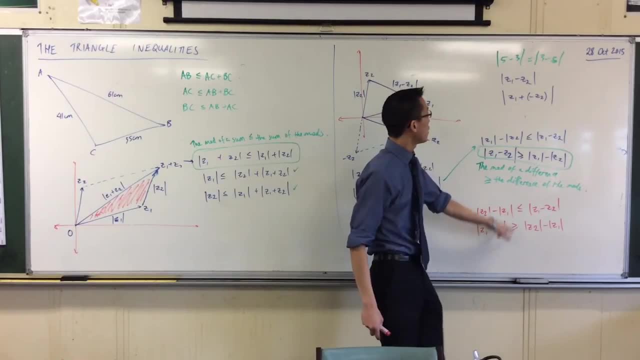 You see, the order doesn't match. I've got 1, 2, and then I've got 2, 1, except for the fact that do you remember we established this before that when you think about absolute value, right? 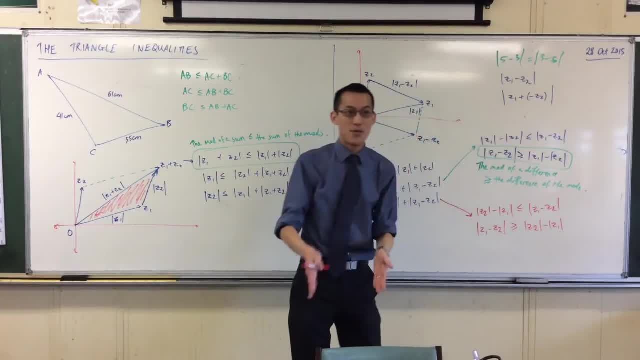 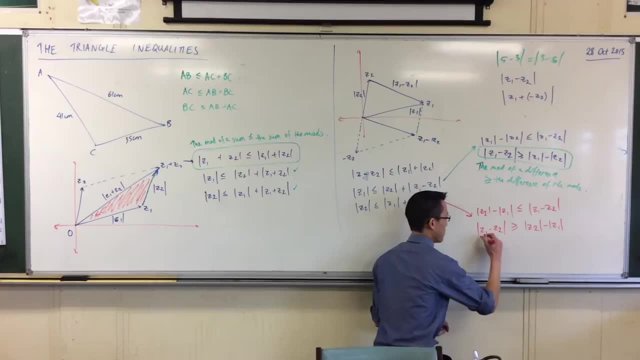 The order in which you subtract things doesn't matter. if you're taking the absolute value, because it's just a distance, It's always going to be positive. Does that make sense? So therefore, this guy down here is really the same as this. 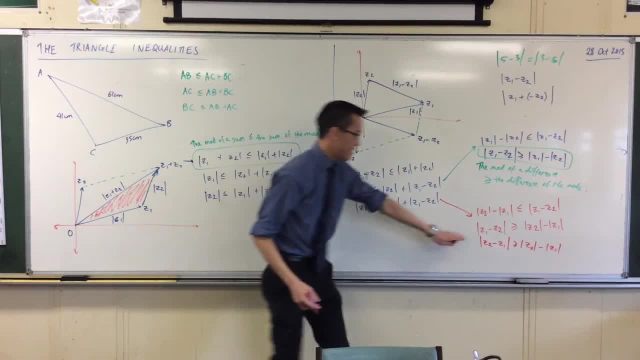 So now I actually do have the order That I want. In fact, this statement is exactly the same as this statement, It's just that I've just switched my labels around: 1 is 2 and 2 is 1.. 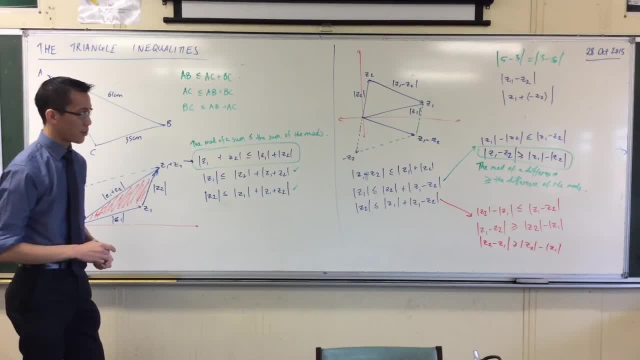 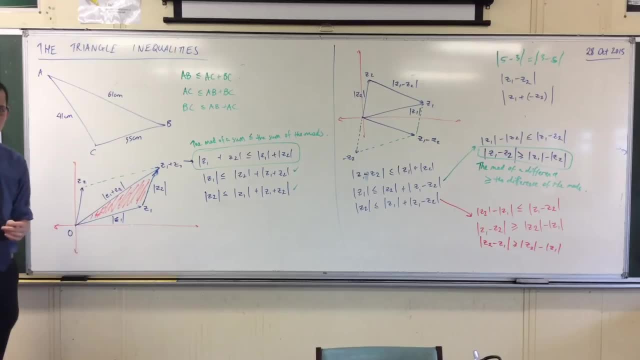 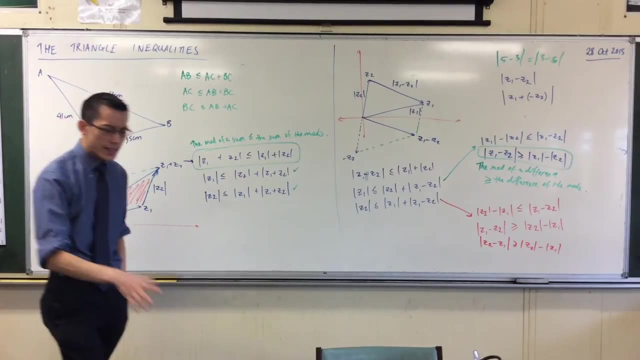 It's the same inequality, okay, Alright, so excuse me, I think that is what will cover this lesson And I'll wait until period 2 to go a little bit further. I guess the thing I would highlight is: I want to highlight two things before you dig into exercise 1.3 a little more. unless you want to do it again. I guess the thing I would highlight is: I want to highlight two things before you dig into exercise 1.3 a little more. unless you want to do it again, I guess the thing I would highlight is: I want to highlight two things before you dig into exercise 1.3 a little more. 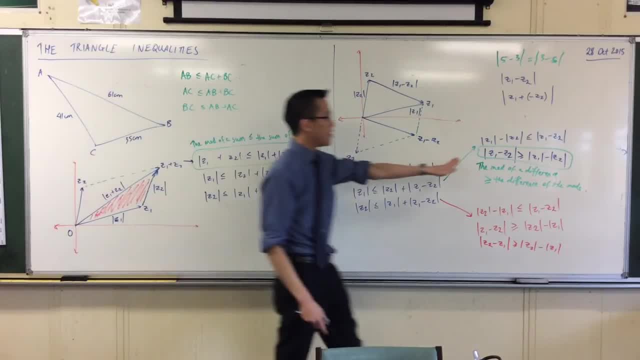 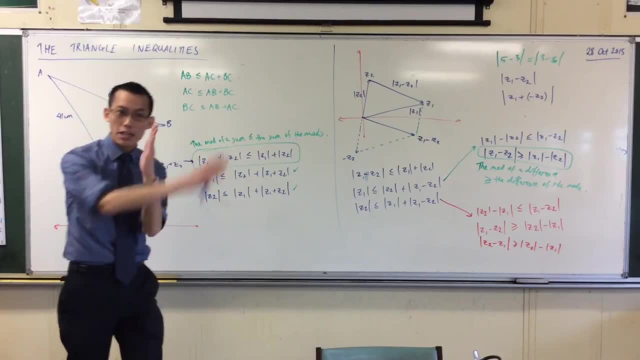 unless you want to do it again. Number one: see this z1 plus z2 and this z1 minus z2 business right. Last time we saw how that was something you could take advantage of in a parallelogram, That the diagonal is a parallelogram, right. 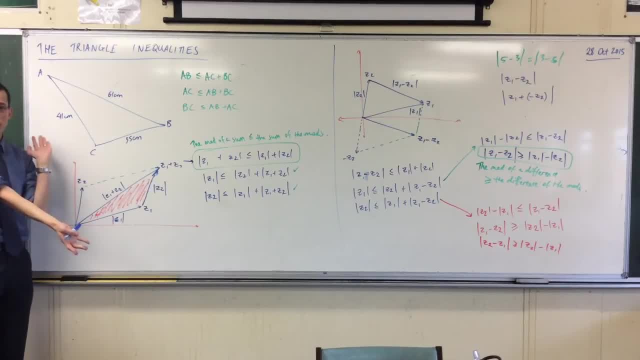 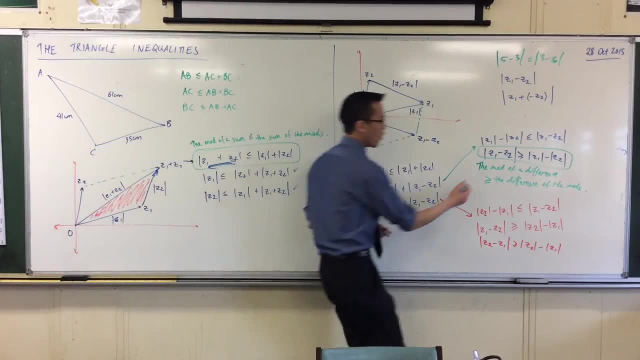 Now we've seen that you can form triangles with these things. So anytime you meet a question which has complex numbers and you see z1 plus z2 or z1 minus z2, that's kind of like a dead giveaway that you should be making some kind of geometric argument.